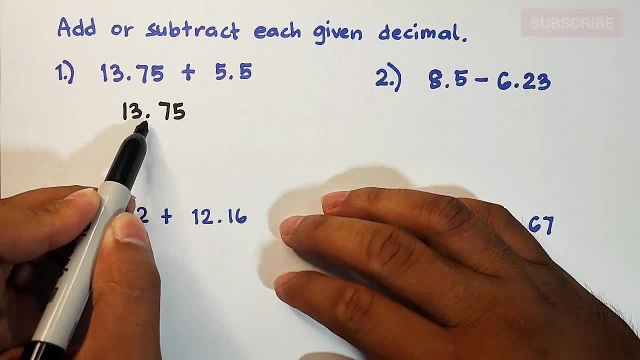 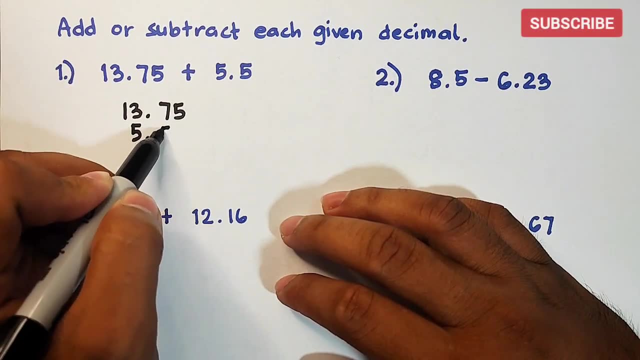 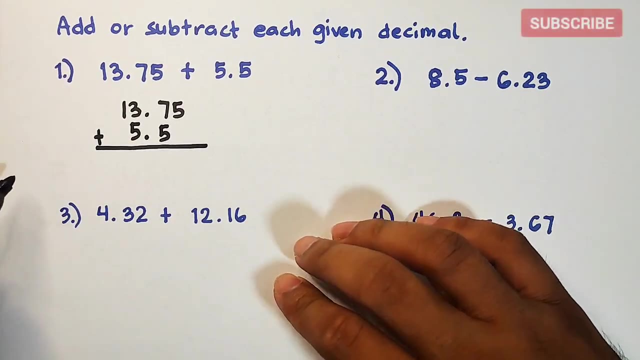 From the first decimal, so we have to align this one. We have this point. Then copy 5 and 5. So as you can see, the decimals are aligned in vertical form 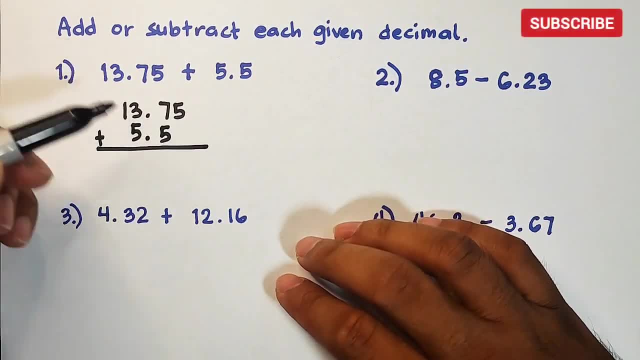 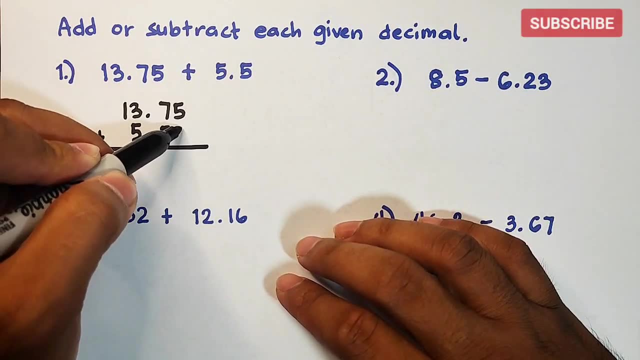 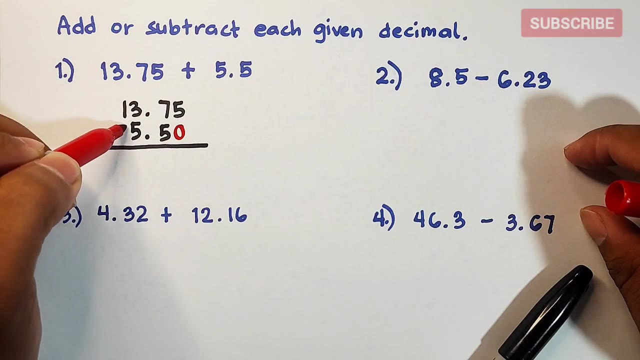 and their decimal points are also aligned. So as you can see, there are holes here or blank space here. So what we need to do is to fill in zeros. So we have to put zero here. So I will use a different marker. You have zero. And here, we can put zero here. So we can add all the digits. So let's start adding them. 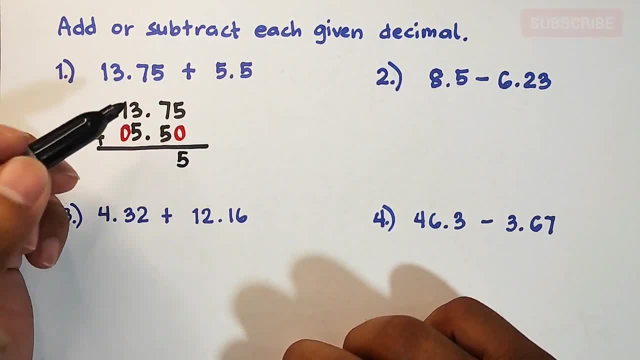 5 plus 0 is 5. Then 7 plus 5 is 12. So we have to put 2 here and carry 1. 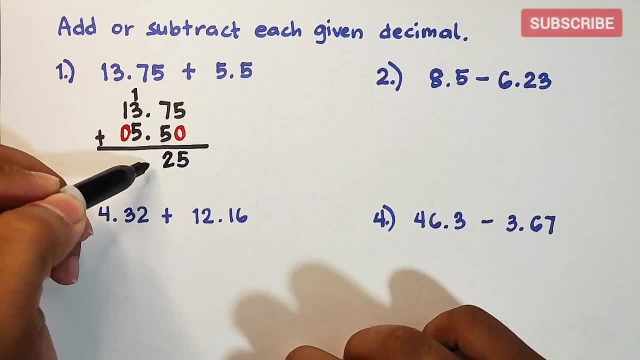 So before adding these numbers, you need to bring down the decimal here. And you can add these numbers. 1 plus 3 plus 5 is equal to 9. 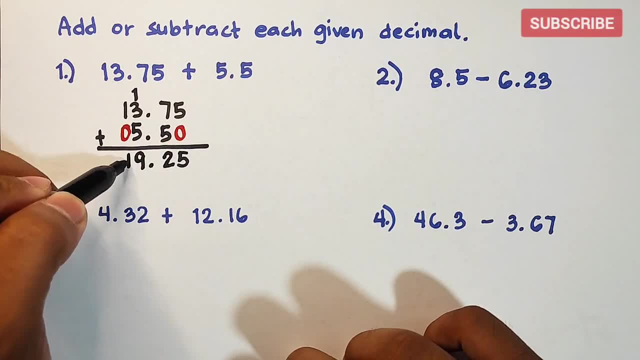 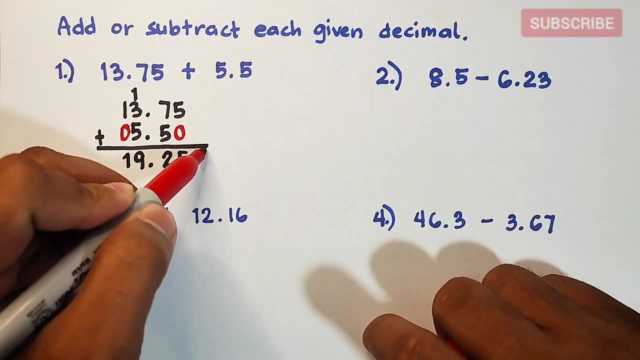 Then 1 plus 0 is equal to 1. And as you can see, the final answer in our first given example is 19.25. 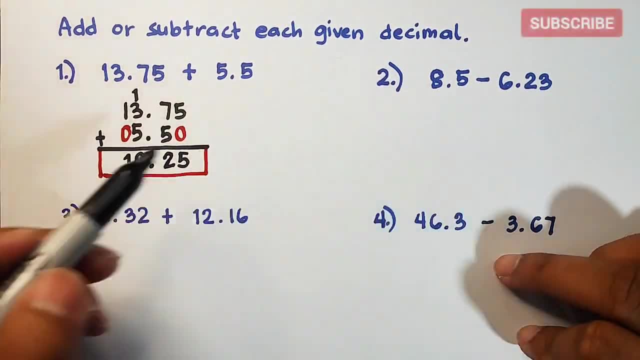 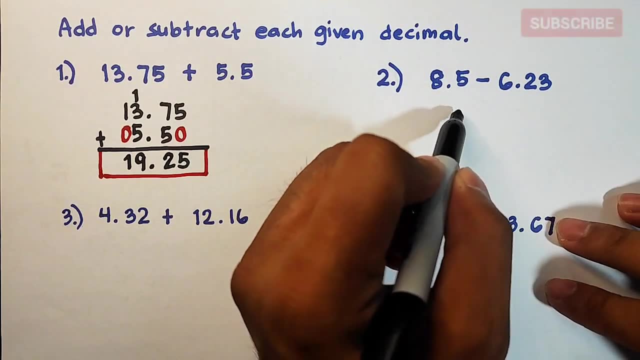 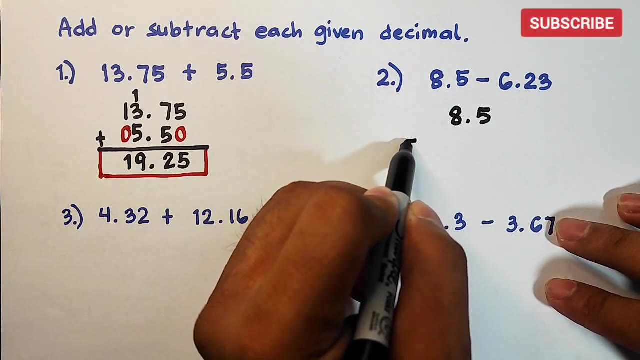 In number 2, we have 8.5. Minus 6.23. First, we need to align them. This one is subtraction. Copy 8.5. We have 8.5 minus 6.23. 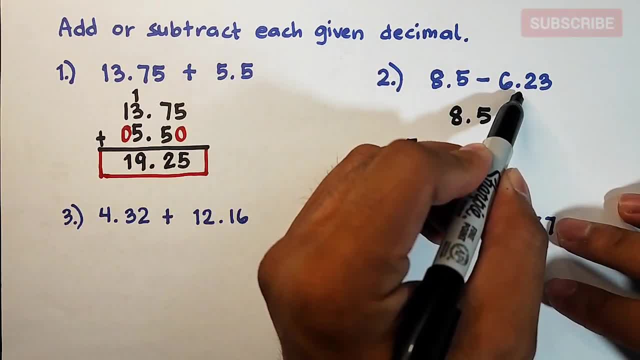 Same thing with addition. We need to align their decimal points. So that is 6.23. 6.23. 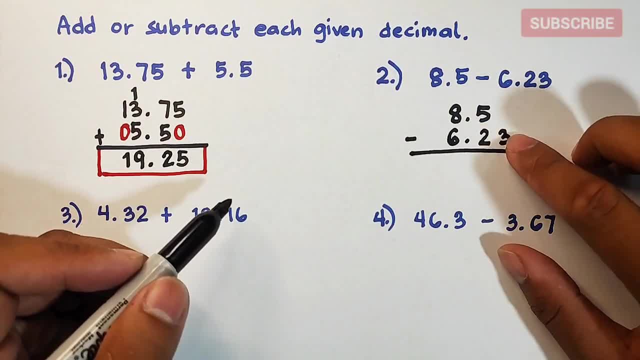 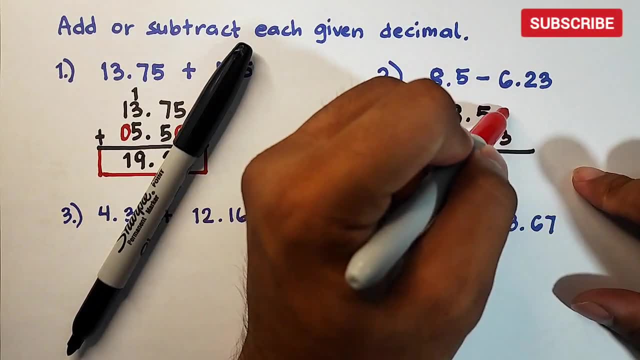 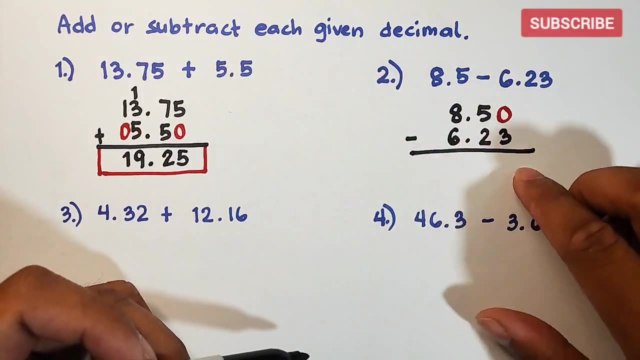 So we need to subtract them. But before that, if you will notice, there is a blank space here at the top of 3. Meaning, we need to fill in 0 here for us to formally start subtracting these decimals. So let's try. 0 minus 3 cannot be. So we will borrow 1 from 5. So it will become 4. 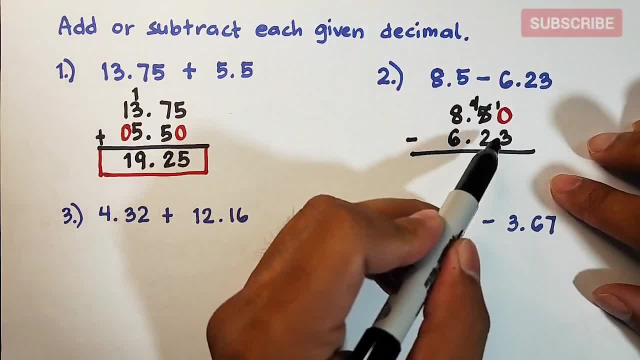 And we will put in 1 here. And it will become 10. So 10 minus 3. Is equal to 7. 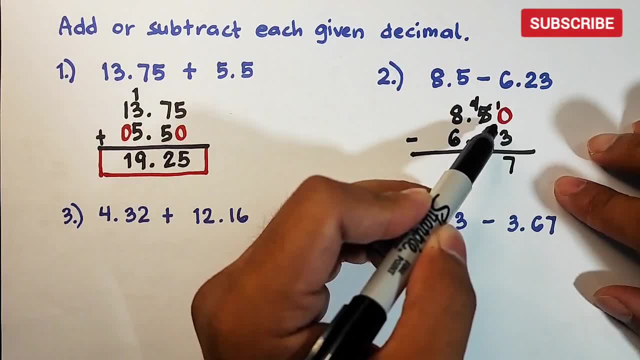 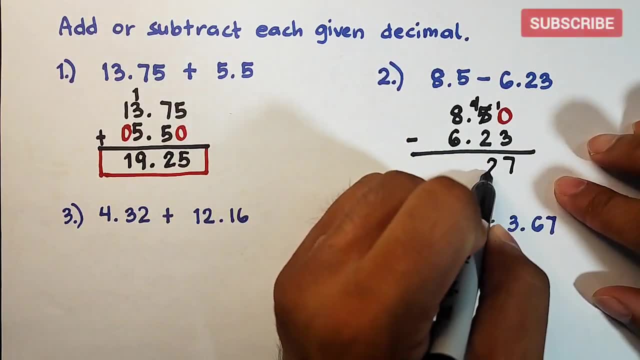 So what we have here, since we borrowed 1 from 5, it became 4. So we can subtract them. 4 minus 2 is equal to 2. Then bring down your decimal or copy your decimal here. Then subtract the last numbers. 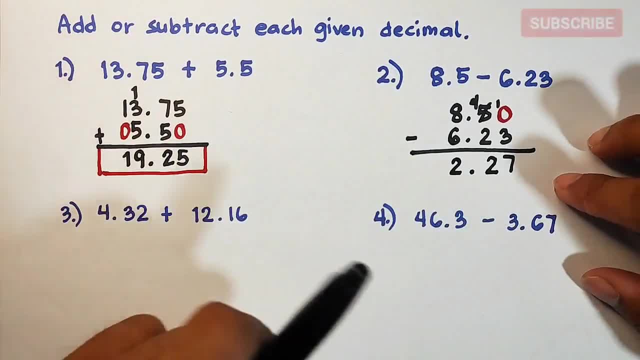 8 minus 6 is simply 2. So as you can see, the final answer in item number 2 is simply 2.27. 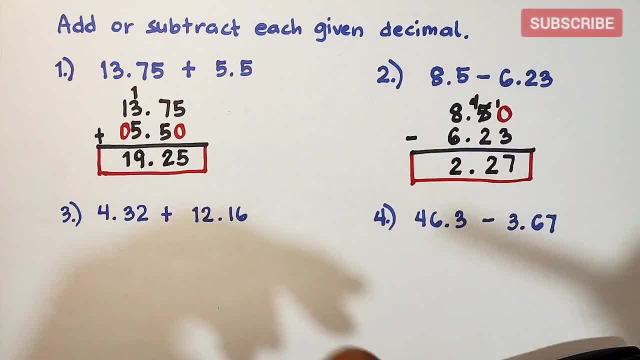 So for others, this kind of stuff are very easy. But for those students who are struggling here, I hope you will learn something from this video. 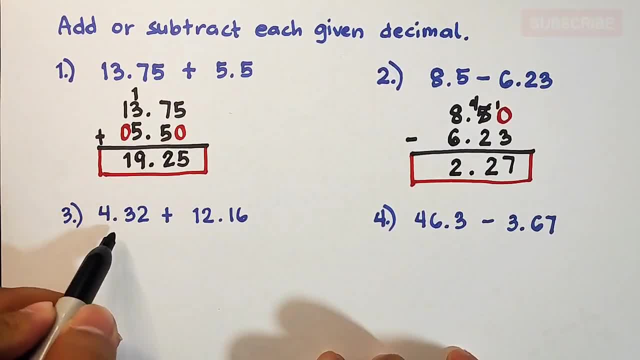 Let's continue with item number 3. For number 3, we have 4.32 plus 12.16. 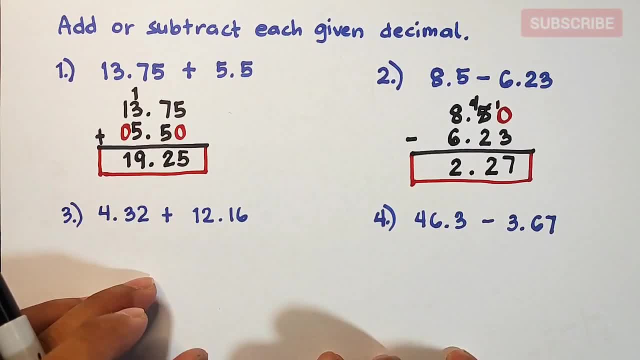 If you want to pause the video and try to answer this, you can do that. Okay, you can pause the video. So I will continue. And later. You can check your answer whether it's correct. 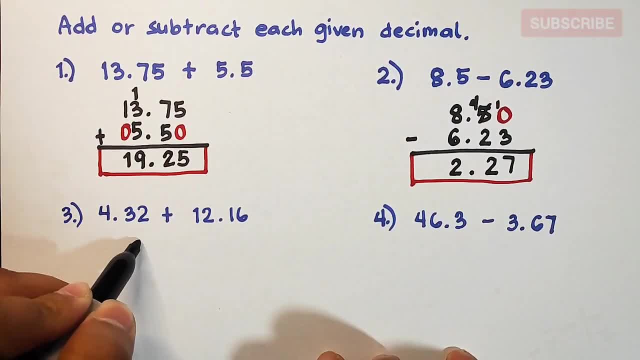 So we have 4.32. 4.32 plus 12.16. So this is your decimal. Then we have your 12. So the digits are not equal. 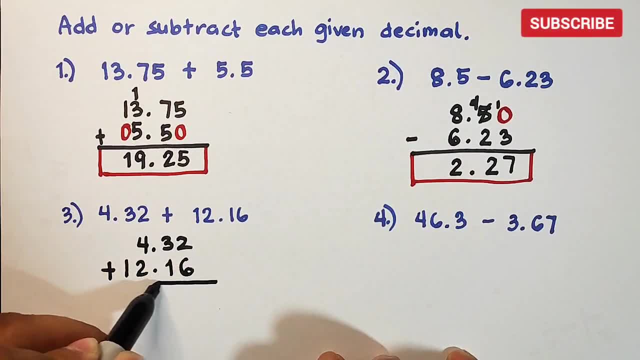 So we have 16 here. So we can add them. 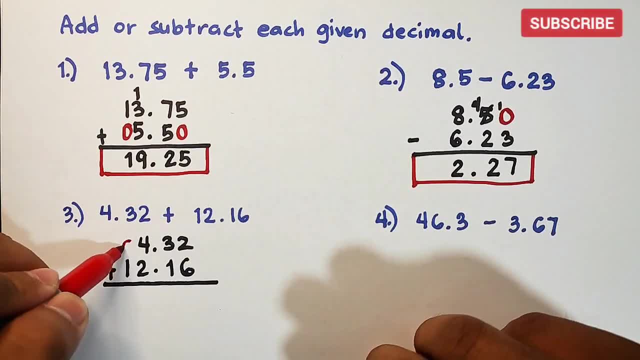 Here, we can put our... Or we can fill in 0 here. So that we can formally add them. So let's try. 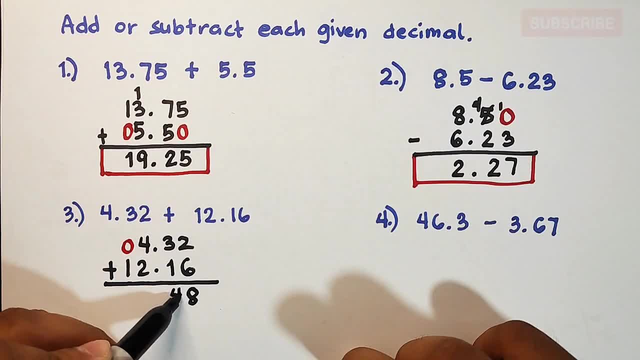 3 plus 1 is 4. Then bring down your decimal. 4 plus 2 is 6. Then 0 plus 1 is equal to 1. 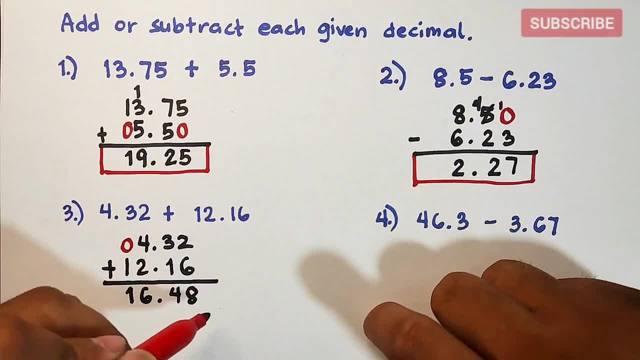 And this is now the answer for item number 3. And this is now the answer for item number 3. And this is now the answer for item number 3. We have 16.48. 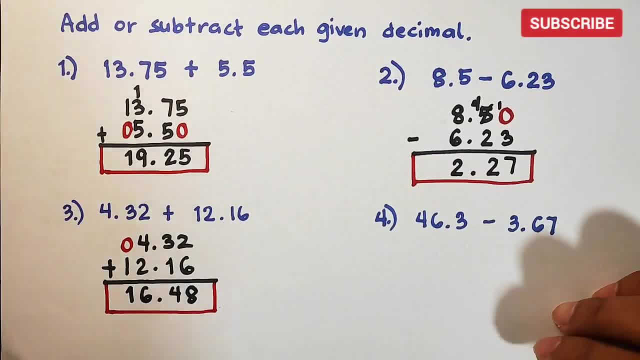 Let's continue with item number 4. And this one is subtraction again. 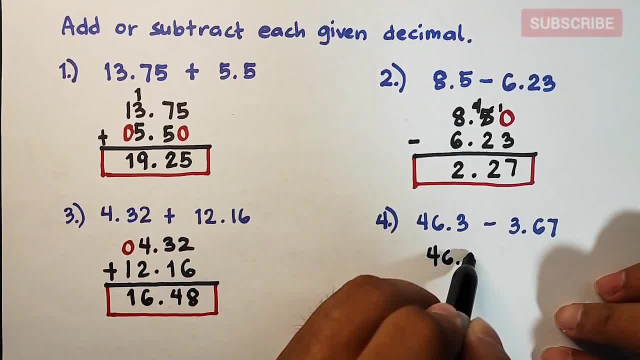 Copy. 46.3 minus 3. Align your decimal points. 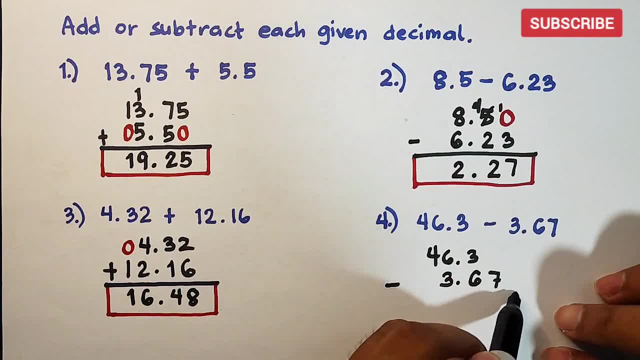 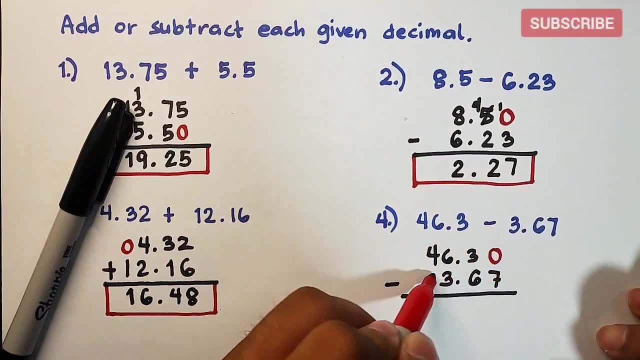 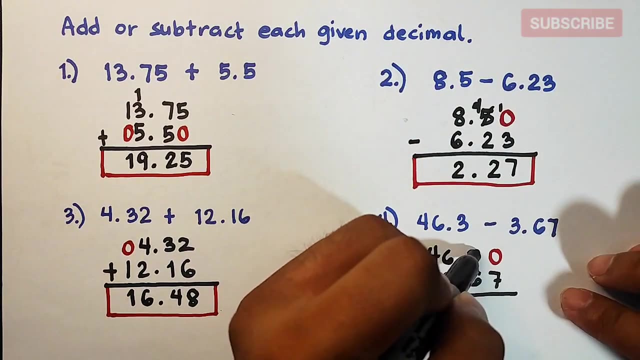 6 and 7. So as you can see, there are blank spaces here. There are blank spaces here. So we need to fill in 0. Here and here. So we'll subtract them. 0 minus 7 is cannot be. So we will borrow 1 from 3. 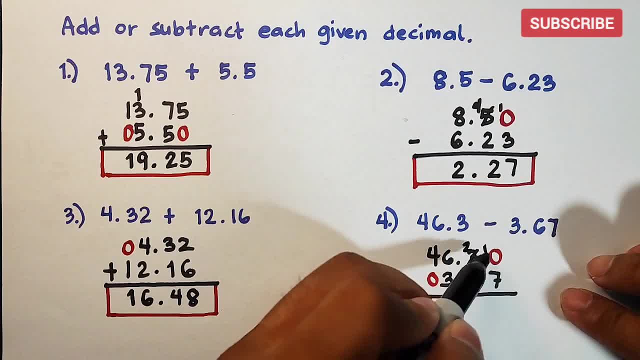 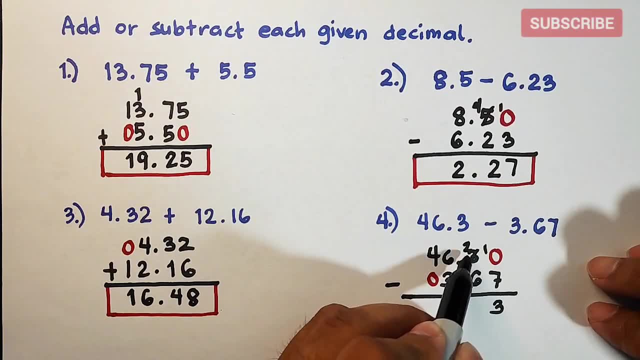 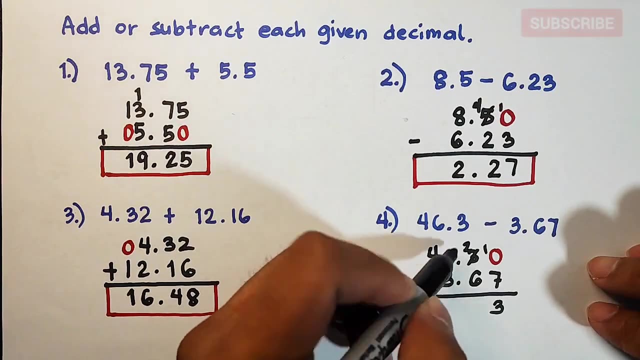 So we will borrow 1 from 3. It will become 2. This will become 10. 10 minus 7 is 3. 10 minus 7 is 3. Subtract this. 2 minus 6 is cannot be. 2 minus 6 is cannot be. We will borrow 1 here from 6. 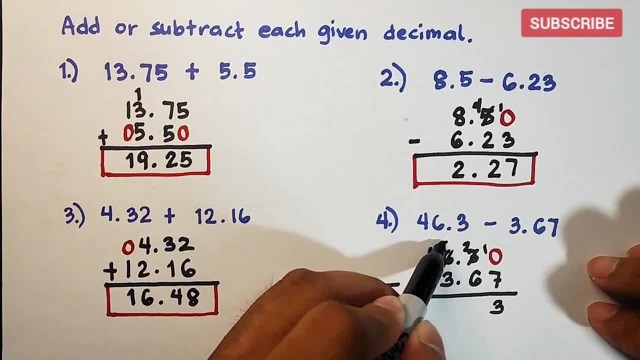 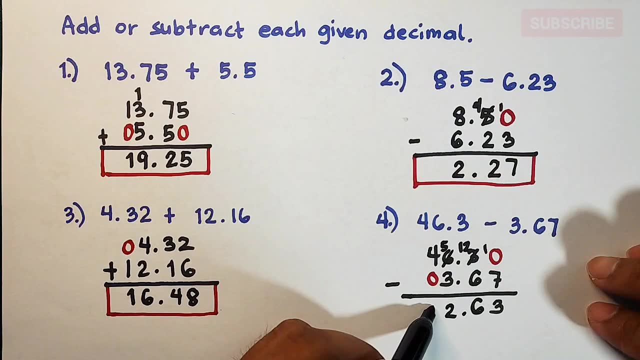 We will borrow 1 here from 6. It will become 5. And this will become 12. 12 minus 6 is 6. Then copy your decimal point here. Then copy your decimal point here. 5 minus 3 is 2. Then 4 minus 0 is 4. Then 4 minus 0 is 4. 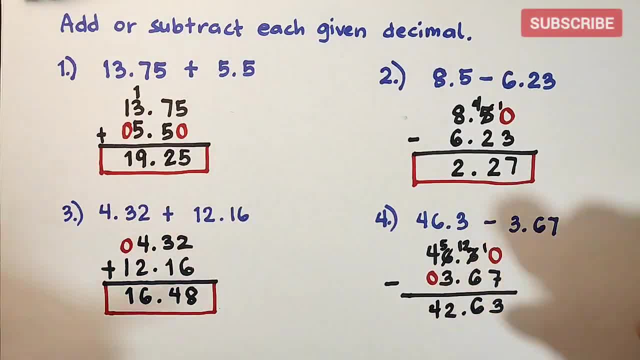 So here is the answer for number 4. So here is the answer for number 4. So I hope guys you learned something from this video. 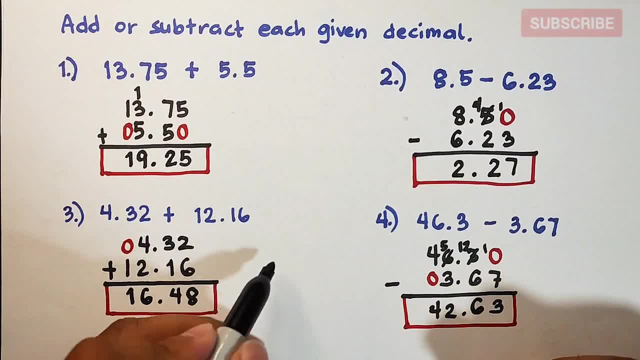 Let's try. You can try this example for number 5. 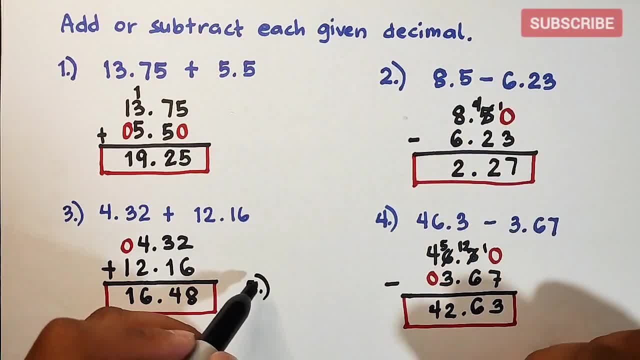 This is your assignment guys. I hope you will answer this. You can put your answer in the comment section. We have 2.1 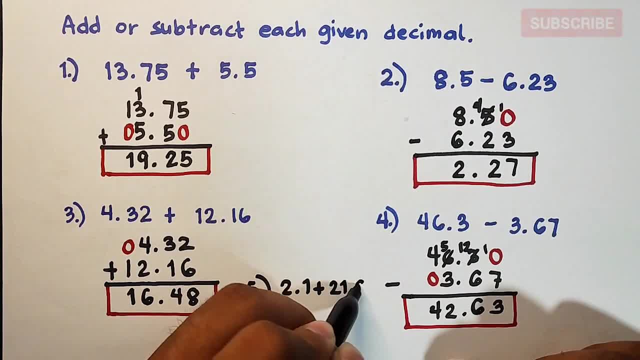 Plus 21.83 Plus 21.83 Plus 21.83 Here is the given guys. 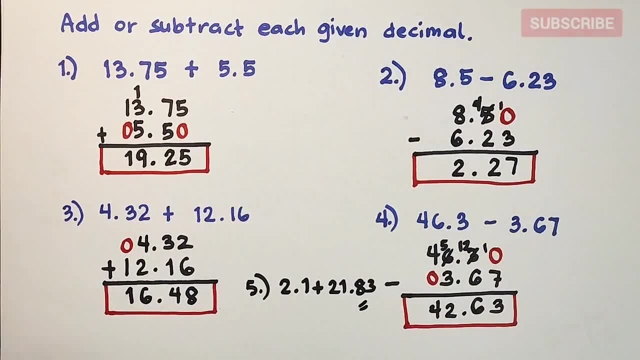 So I hope guys you learn something from this video if you're new to my channel Don't forget to Like and subscribe but he hit my name Bob button for you to be updated satin latest uploads 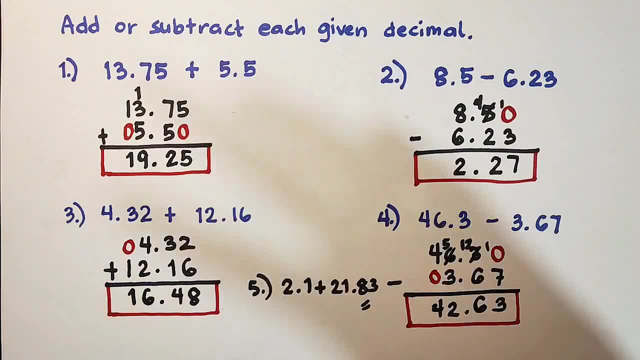 Again, it's me teacher gone Marama Marama Salamat Bye. Bye 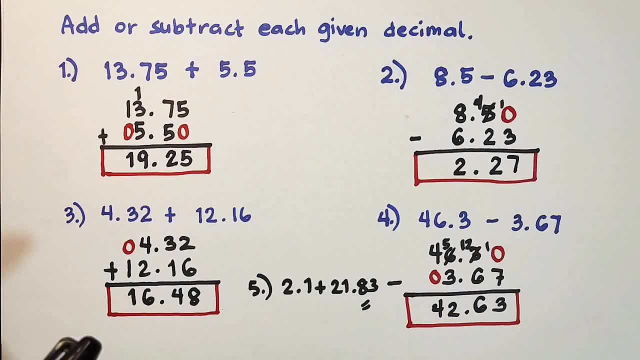 By the way guys, I will put the link of the other videos about decimals in the description box. So, thank you